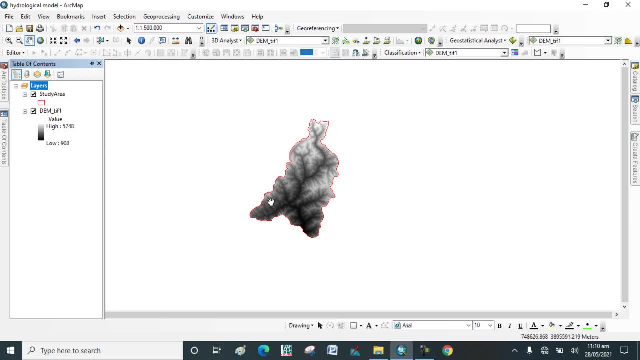 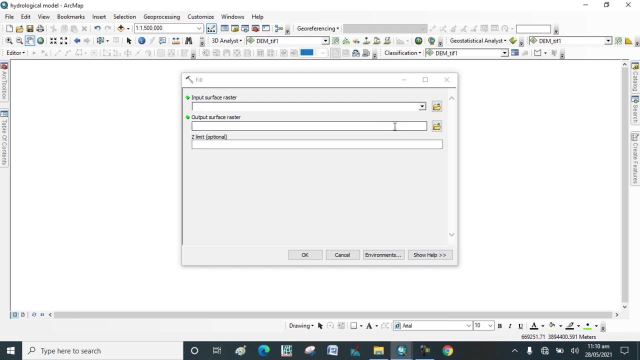 So we are going to start. First we are going to our toolbox and go to specialize tools and hydrological tool and find fill of the study area- here is hydrological tool- and click on fill and which surface raster? click them on study area. note that you must noted the output location of your study of the 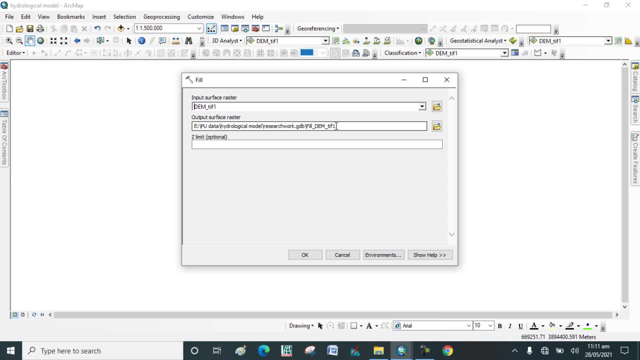 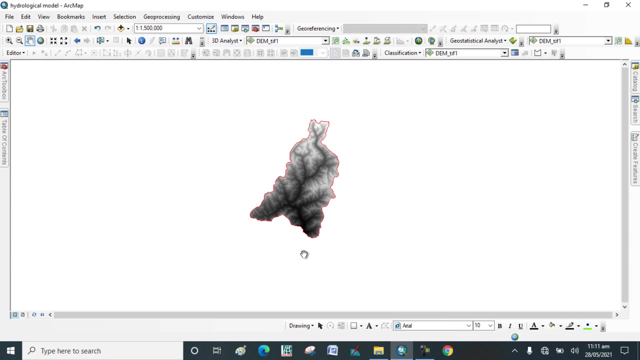 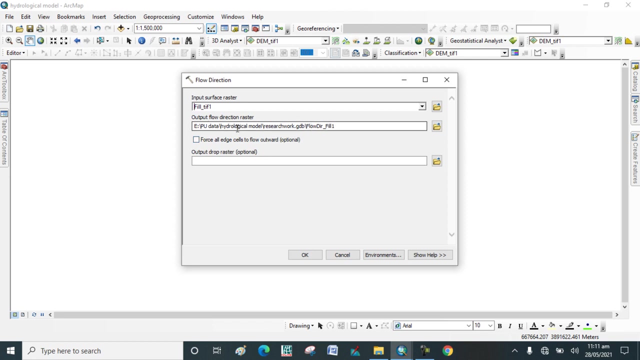 fill or output file, because you will need it for further work. so click on okay, wait for the results. now fill map is marked. now go to again and prepare flow direction map and flow direction input surface raster is fill. we will add there fill and here you must know that where is your is output location. so this is the flow 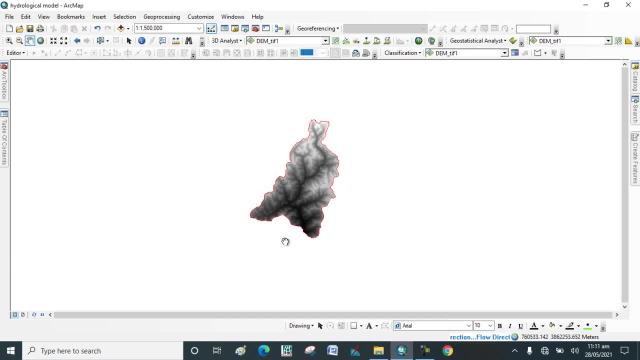 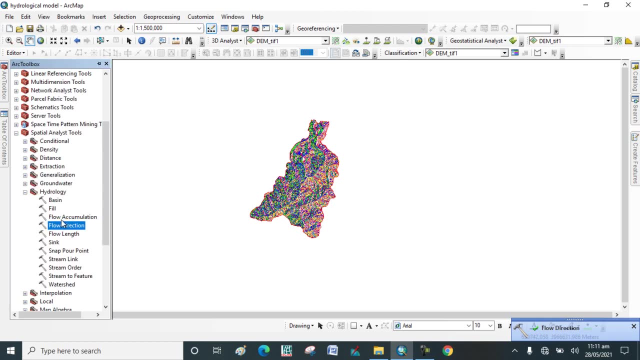 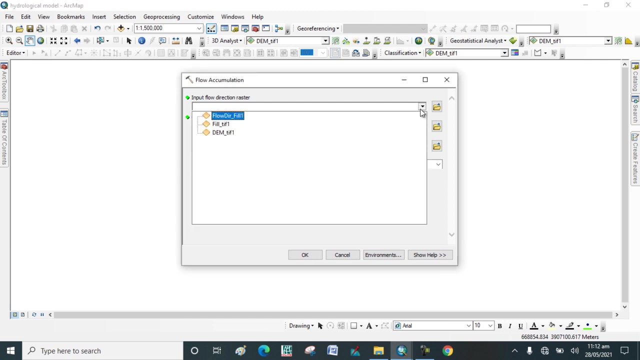 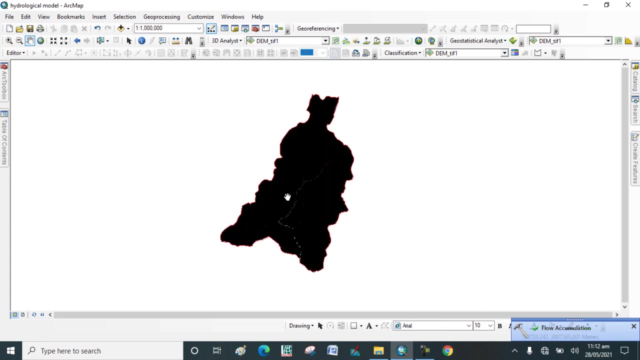 direction. after that, again go to raster. sorry, again go to our toolbox and click on flow accumulation, flow accumulation. he added input: flow direction, raster. here we will add the flow direction and here you can see that the flow accumulation. okay, you wait for the results. now the flow accumulation map is prepared. you can see. 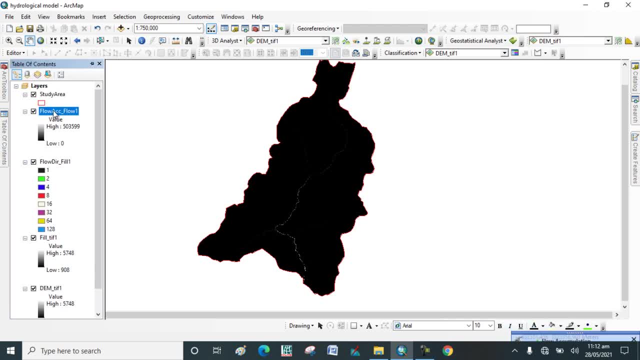 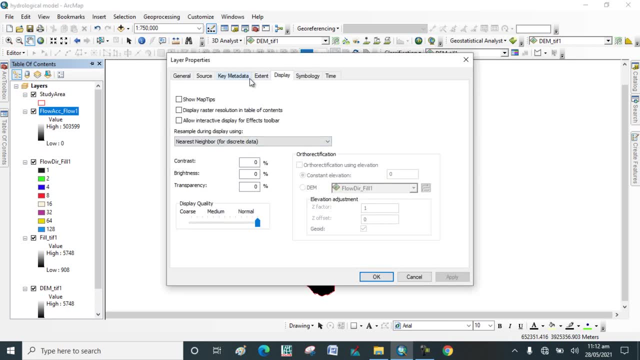 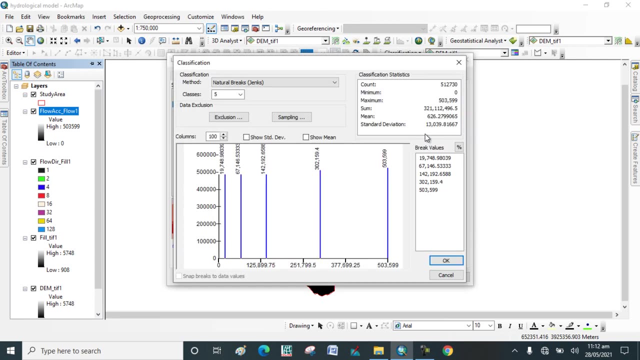 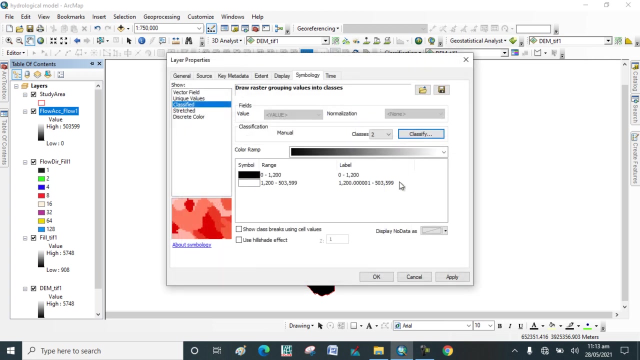 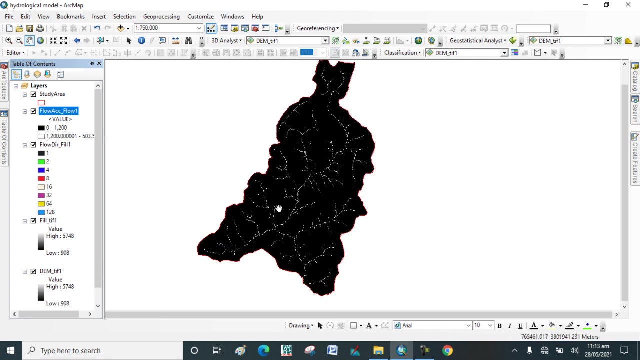 that go to table of content and go to properties of flow accumulation. here you can go to symbology and classified, classified date and two classes, and you can add the upper break value, which is twelve hundred. take an okay, okay and you can see that we classify the flow accumulation map and two classes. 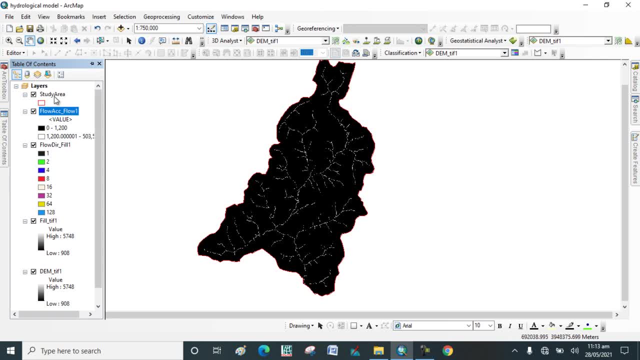 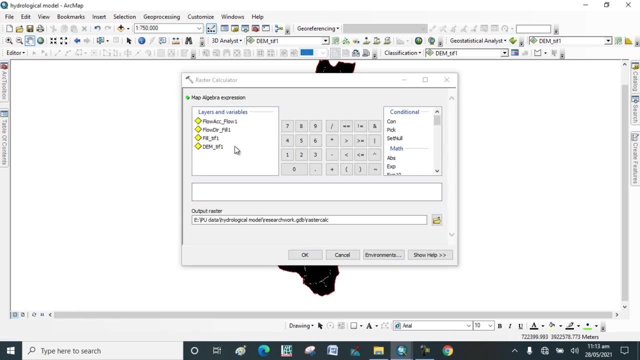 after that, go to map algebra tool and out toolbox- here is the spatial analysis tool and here is map algebra tool- and go to raster calculation and type the following formula: flow accumulation as greater than 1200. now, ok, here give name, element, output, raster class, case, flow direction. that is all. now wait for the result. Dir Man места classWhen 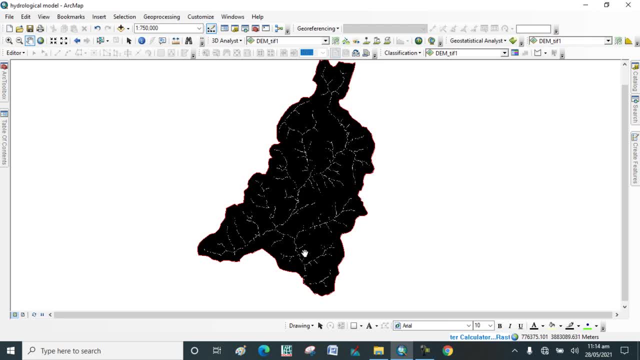 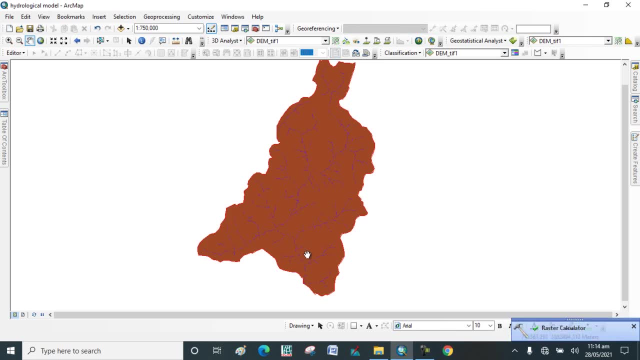 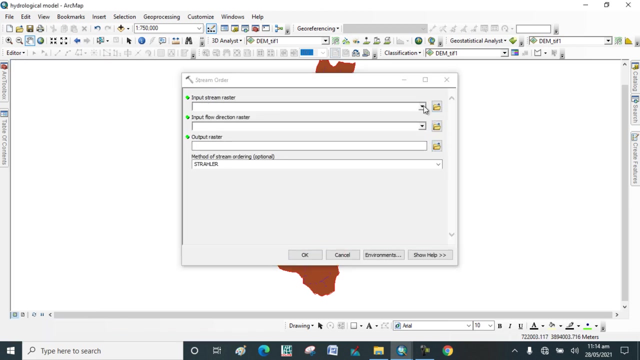 Time Minuten lict my Result: cinqu reading qx1 net end. now go to R toolbox and go to to hydrology tool again and prepare the stream model map. here we can add the raster calculation of flow accumulation, which is calculated now this one- you can see that that one- and output flow direction. here we can add the flow. 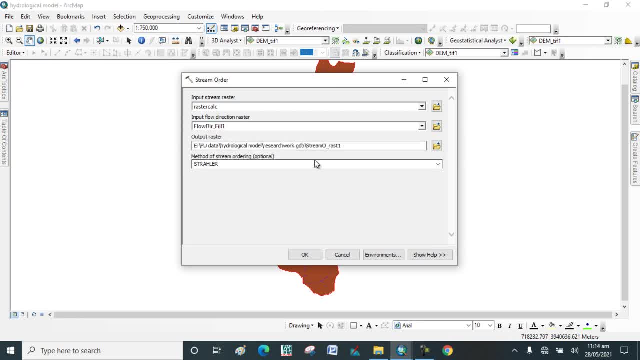 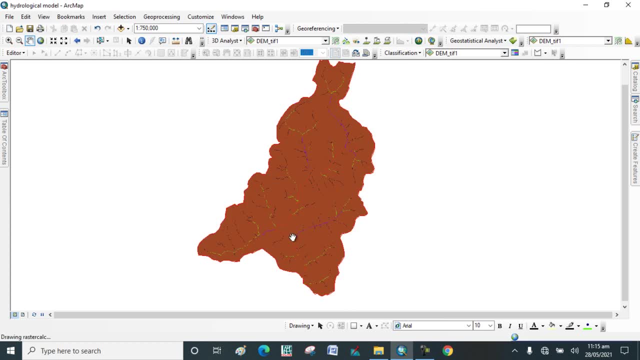 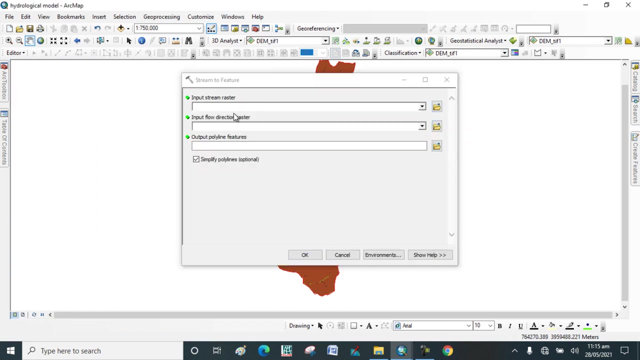 direction map, which is that one now click on ok, this is stream model map. after that it is classified into four classes. now go to stream to feature tool. in stream to feature tool, we will add the flow direction. ok, here we will add stream order map and here we will add the flow direction. click on ok. 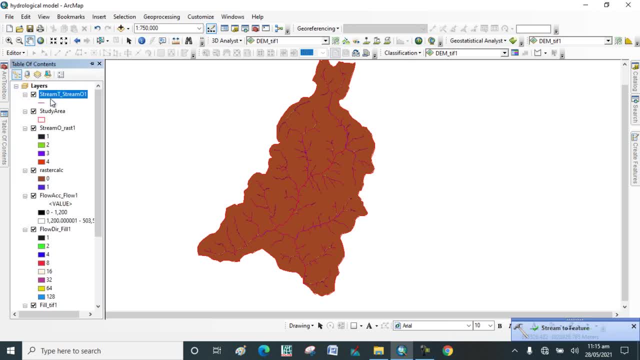 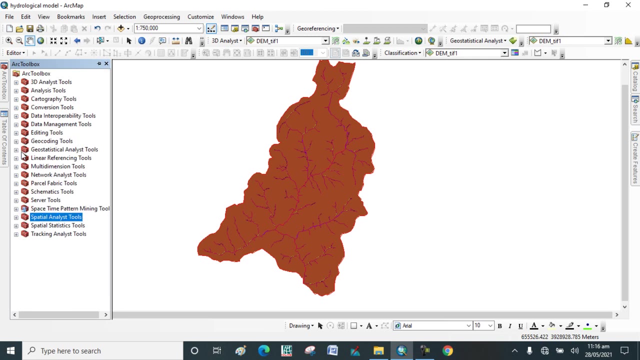 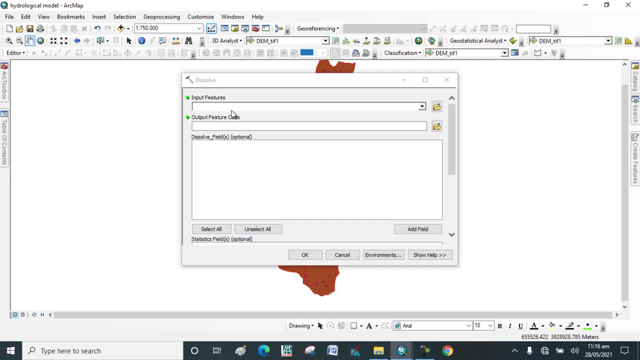 now you can see that the stream to feature map is prepared. now go to data management tool and dissolve this stream to feature. go to data management tool and go to generalization and click on dissolve tool. here in this, all tool will put the input feature is stream to feature, which we make now stream to feature. 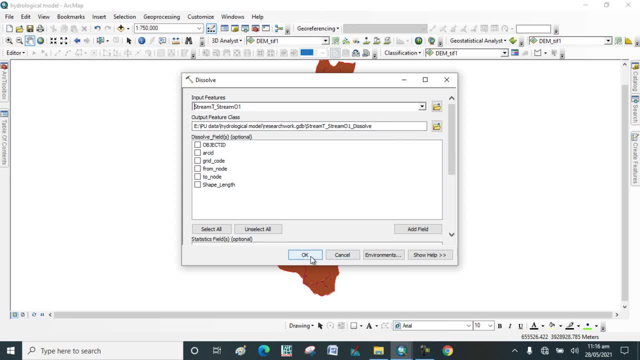 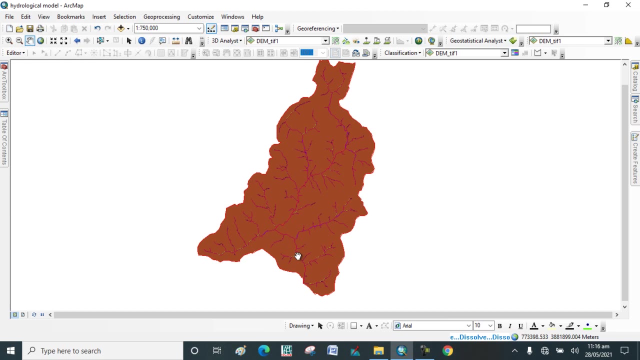 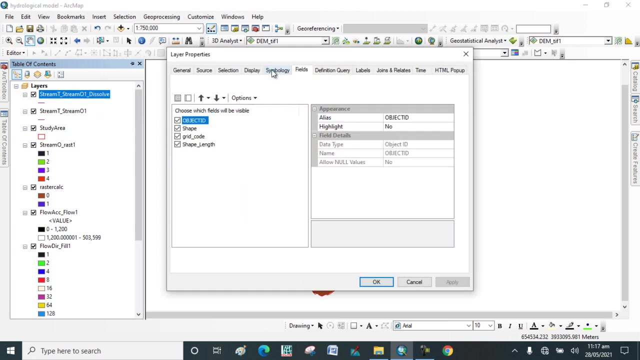 output name is stream to feature dissolve. so, and here we will select the great code. click on yes now. click on ok. here you can see that in table of content the result tool is make. now go to properties of stream to feature dissolve tool. here go to symbology and go to categorize and great code and 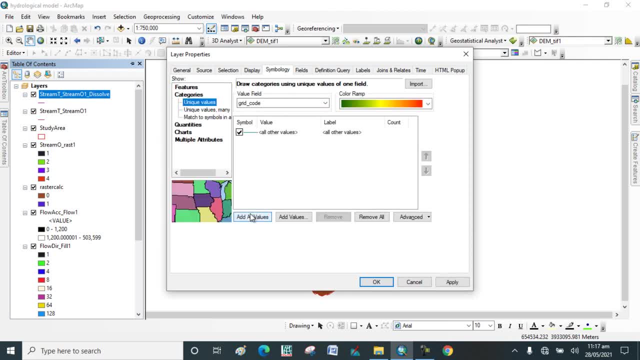 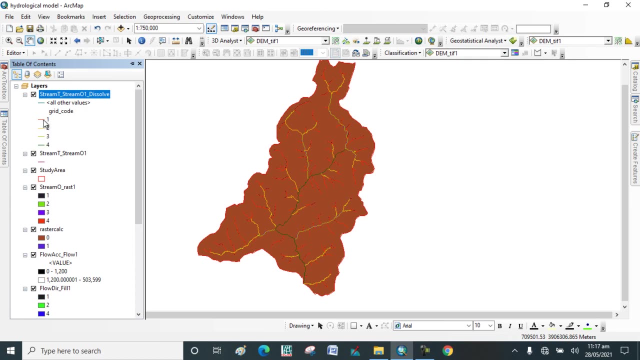 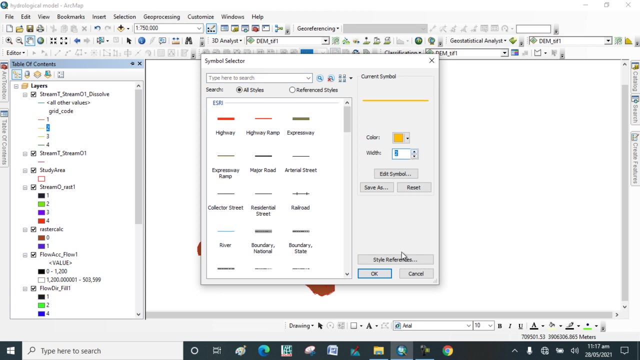 add all values, you can see that it is classified into four classes. so okay. so that's all for this video. thank you for watching. bye, bye, bye, bye. so okay on it now. give it the increase the sizes of the stream to feature. click on ok, you can see that it might clear. now increase the width of third line. third order is three. 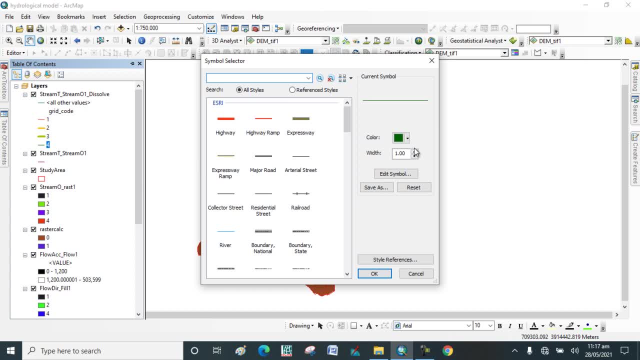 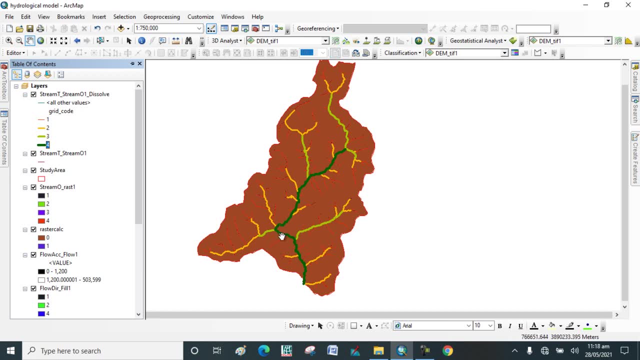 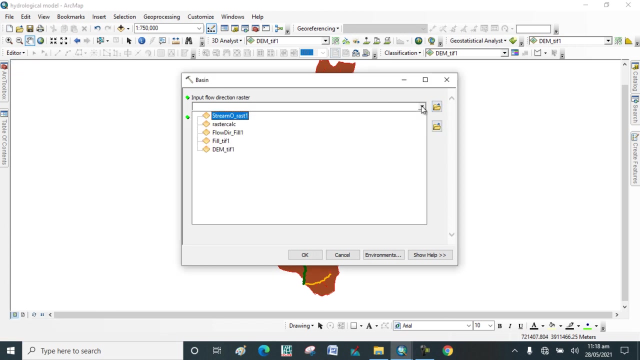 now fourth order, it's might: clear stream order, dissolved stream, first order and second order. this one third order and the green is fourth order, dark green. so now again go to our toolbox and go to hydrology tool again and then make the basin map. total parameters don't exceed ακ. 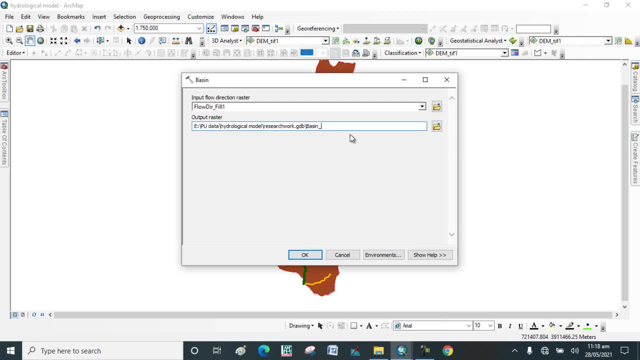 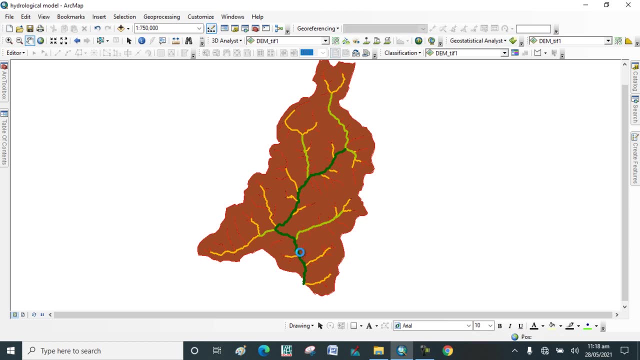 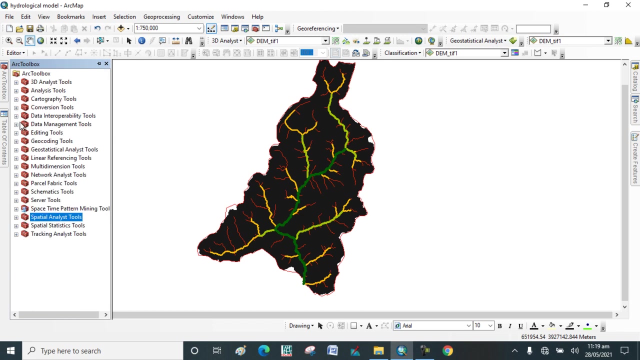 weight so around, creating the Motor flow flow 4000. 100%. now basin is prepared. you can see that it might more clear. so now go to data management tool and reclass the flow direction map or resample it. go to data management tool and data management tool. go to raster tool and raster tool. go to 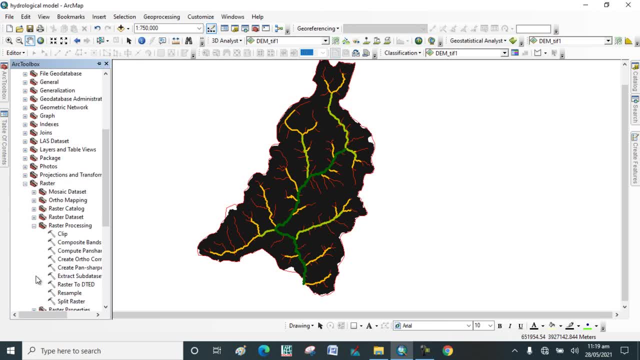 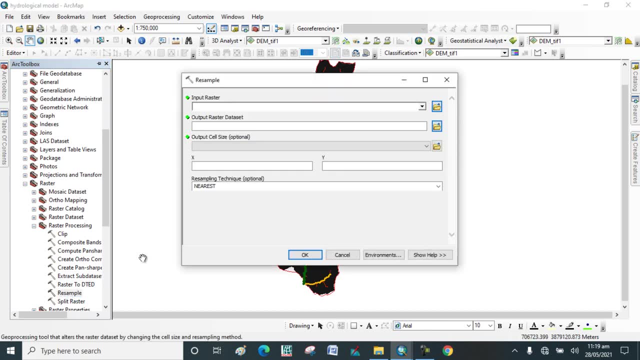 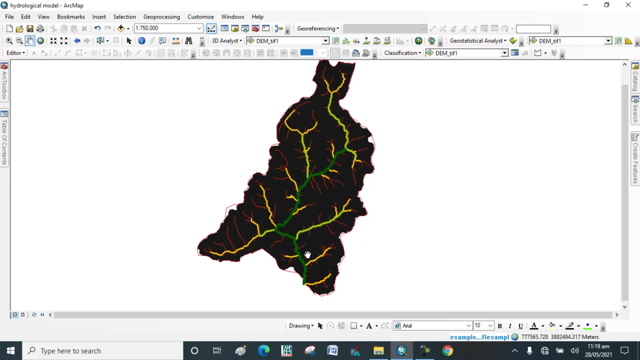 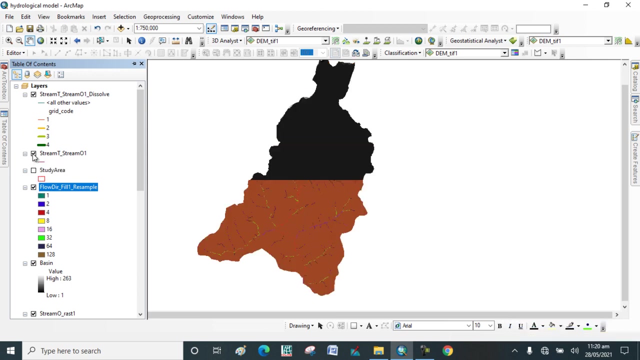 raster processing and raster processing. click on resample tool. resample input is flow, direction is that one. this is resample. now click on ok. why we resample this map? because it will give us the pixel information. if we uncheck this, all value except the resample tool. we uncheck this all value. it will give us the information in pixel. 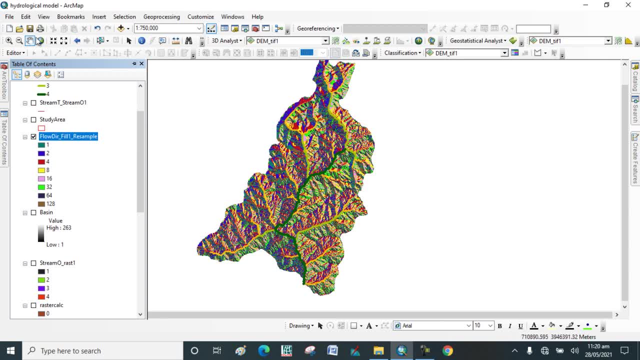 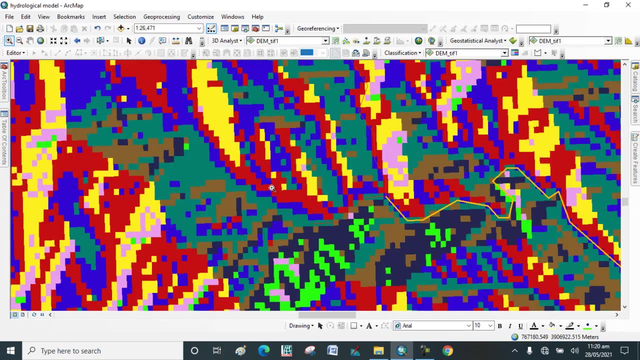 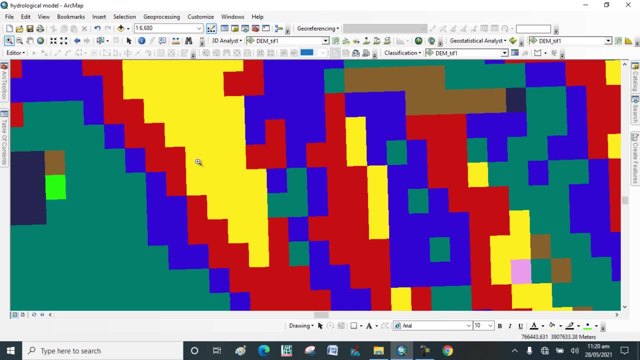 information. it will give the pixel information. so if i take the zoom tool and zoom this map, it will give us the information pixel wise. you can see that this is the pixel information. its gives us the pixel information. for that purpose we apply resample tool on flow direction map. 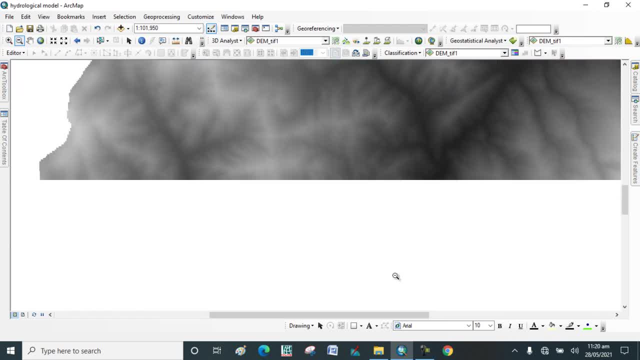 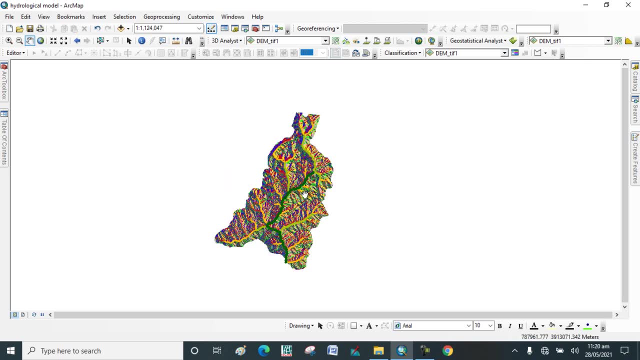 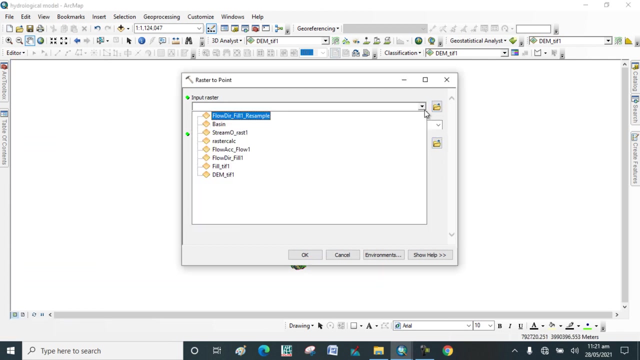 back is zoomout it and further proceed the work. after that we will convert this raster to point. now go to conversion tool and conversion tool. you can see that conversion tool from raster. click confirm raster from raster to point. now, if I select that input, raster is flow. 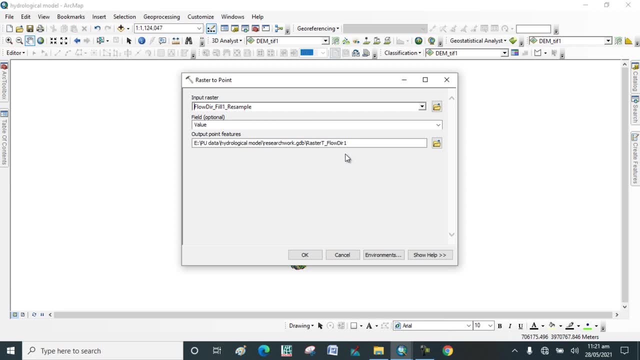 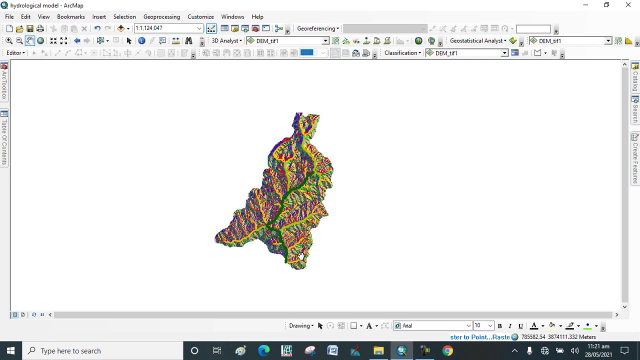 direction to sample. it will gives raster to point. give name it raster to point. click on ok. if uncheck these all except raster to point here, we will see that and check these all. value. now add this, one, add slash, and it is sample to point: raster to point. 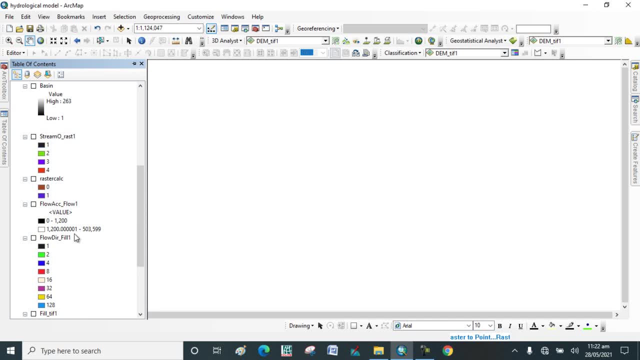 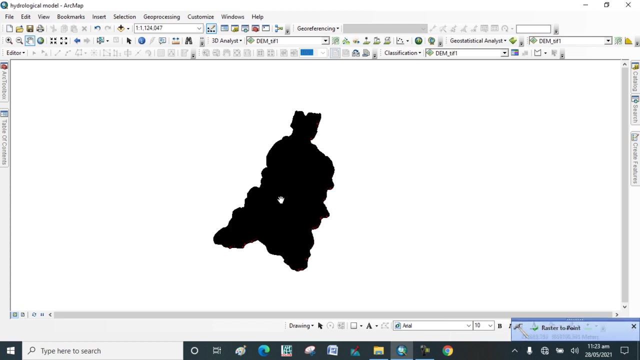 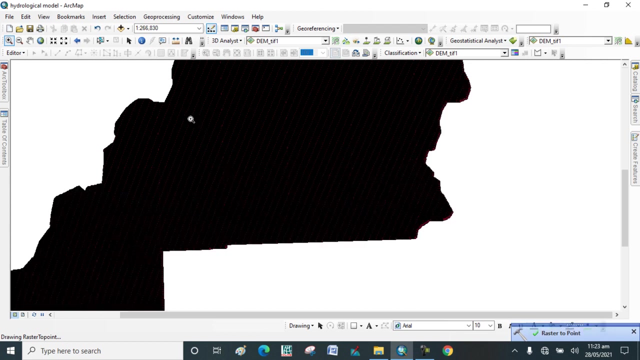 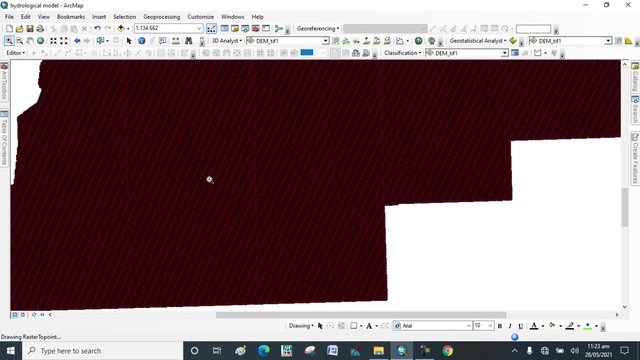 it is raster to point and it is raster to point. Now it's done. it's totally show black in color, but if we zoom it it will give us information about the study area and points. if we further zoom it now, you can see that. 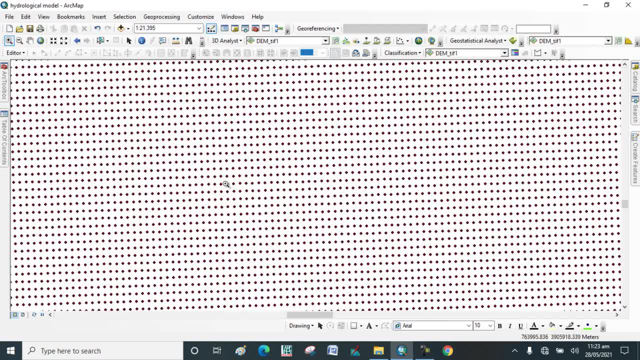 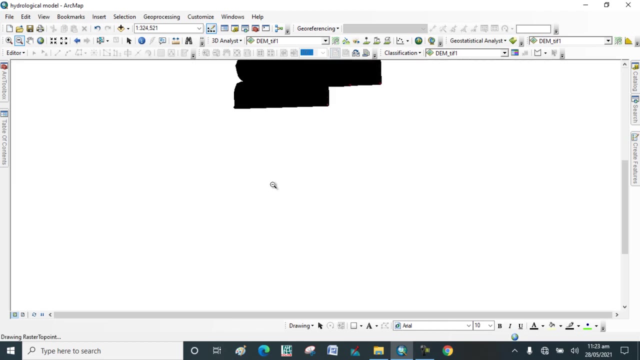 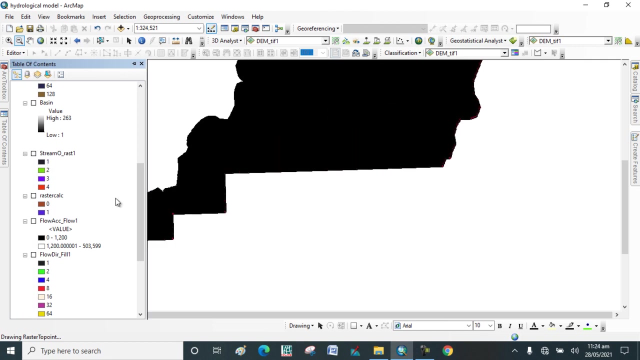 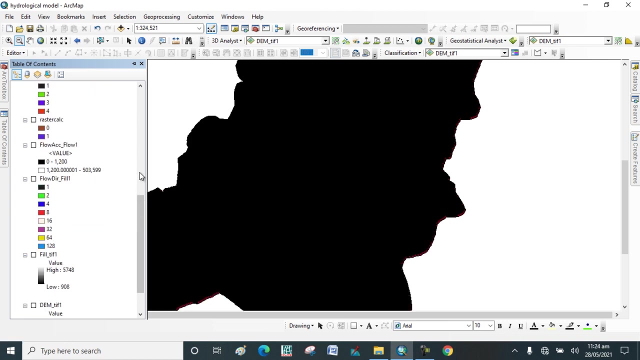 it give us information. really, you can see that it give us information in points. we convert this flow direction resample to points Now, after that We will go to the properties of that and add the unique value of grid code accordingly. So zoom out this and for that it might vary. 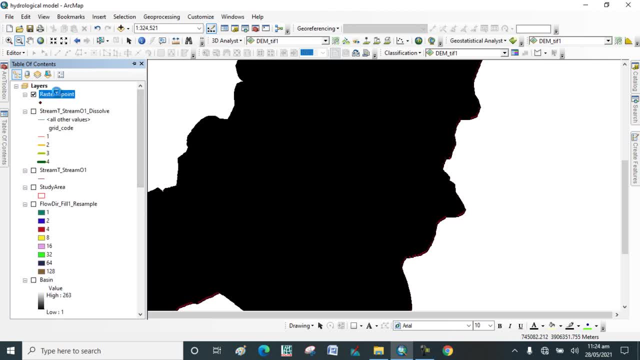 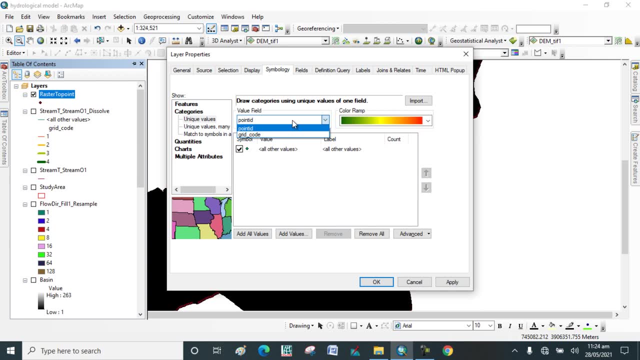 Now Click on properties of that and go to categorize and get unique value of grid code and add our value right for that. Now you can see that it is categorized. Okay, sequence: the angles: We will discuss this in detail and next lecture. 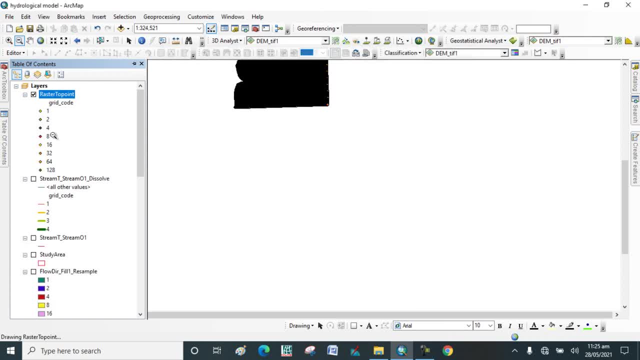 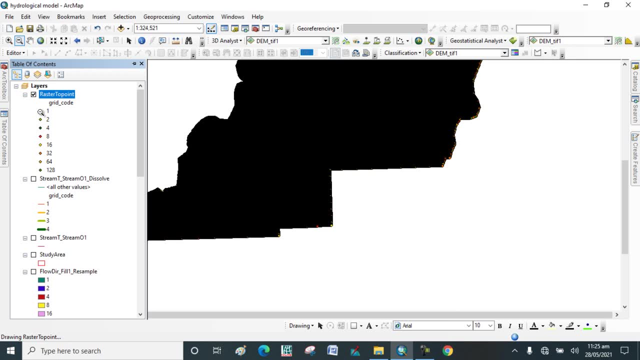 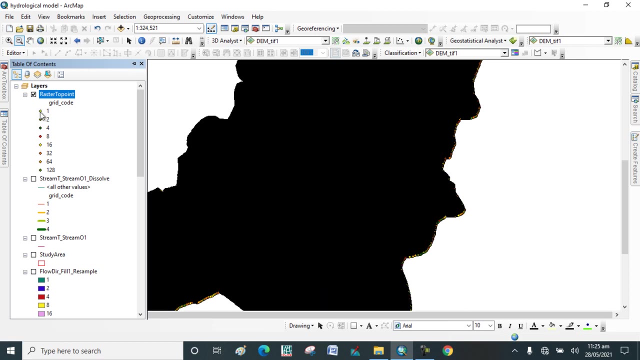 So fill now. I click on ok. you can see that the grid code is this: you change the angle, that one which is equal to 90 degree and two which is equal to 45 degree. Now We will take these will arrange the flow direction and find the flow direction of the study area. so 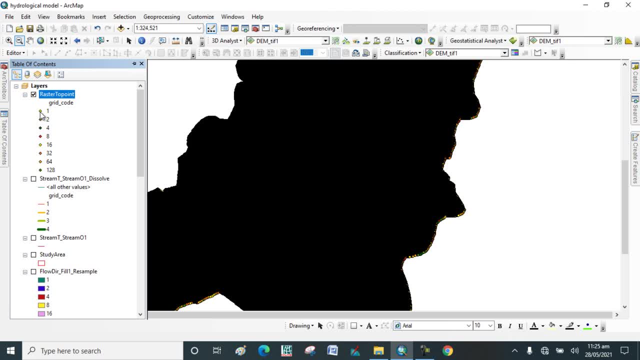 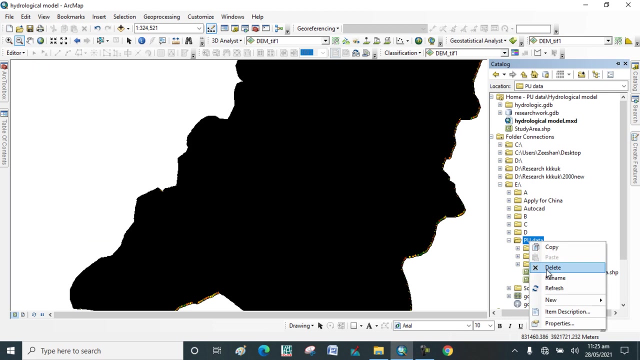 now go to catalog and create a shape file. we are moving towards the hydrological modeling, so for that we required the points of which is known as power point. for that we create a shape file for our study area. go to catalog and search the location where you want to create a shape file and get the name. 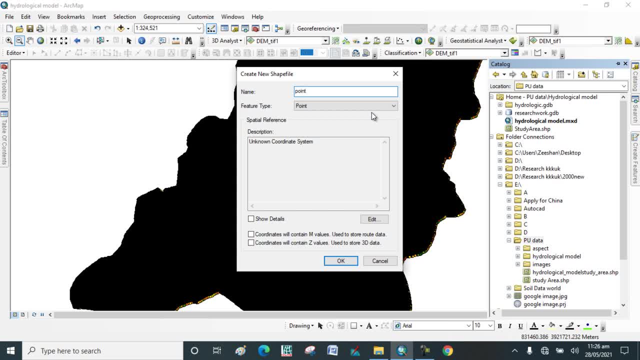 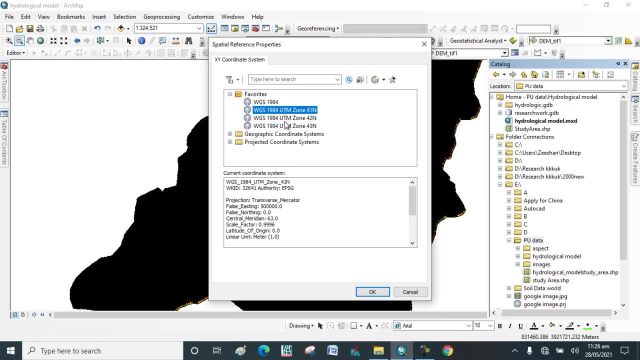 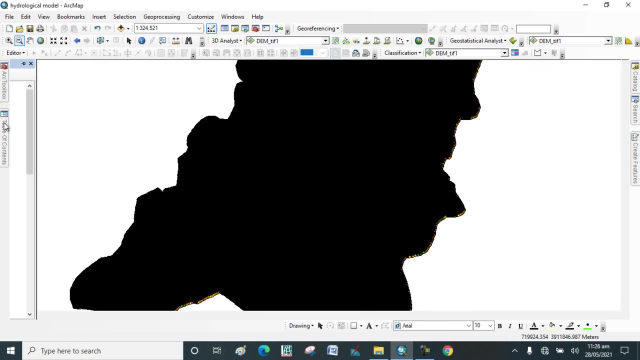 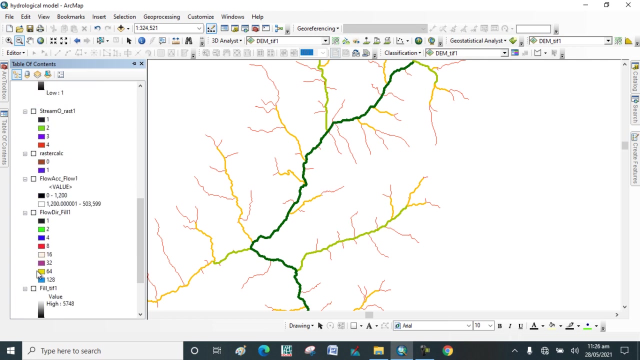 shape file to point and feature type point coordinate system and select your coordinate system. click on ok. ok, now you can see that the point shape file is created. type is point now. after that we are going to uncheck this one and check that one also. study area. 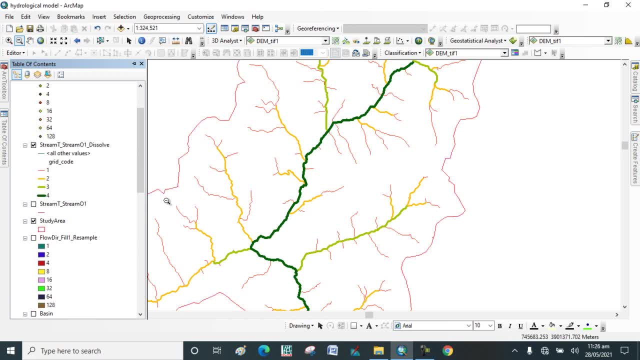 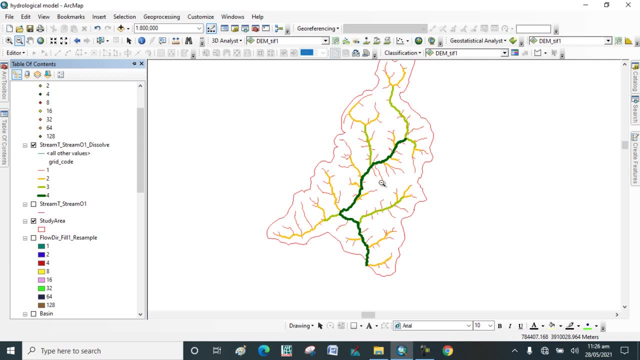 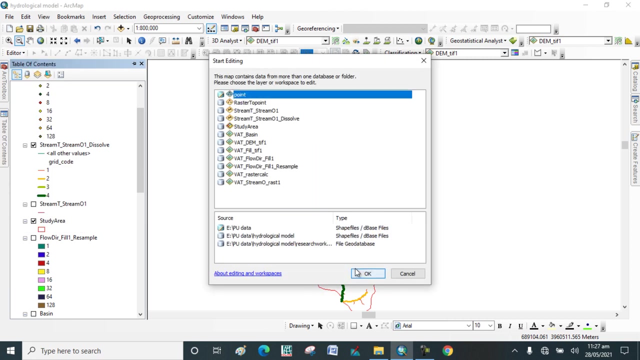 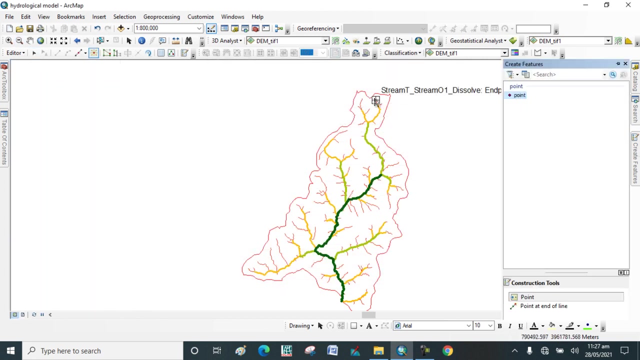 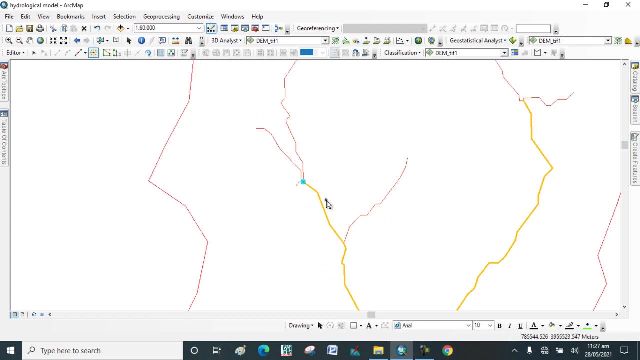 that one is study area map. so now take some point from the edge of the stream, start editing to point. okay, continue, continue, ok, pick the point and mark the point, zoom this stream order and here take the point first and also here: second one, third one, fourth one, third one, fourth one, third one. 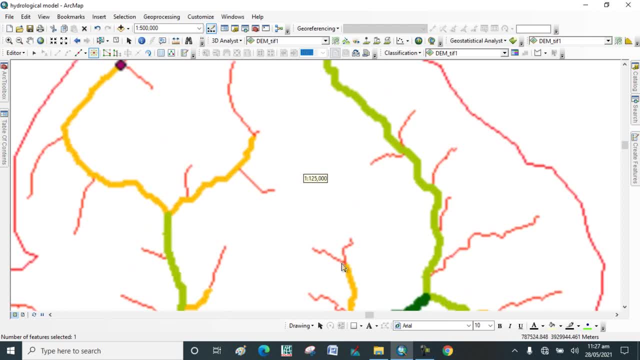 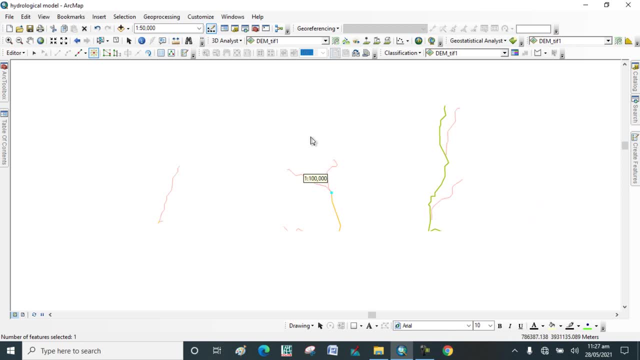 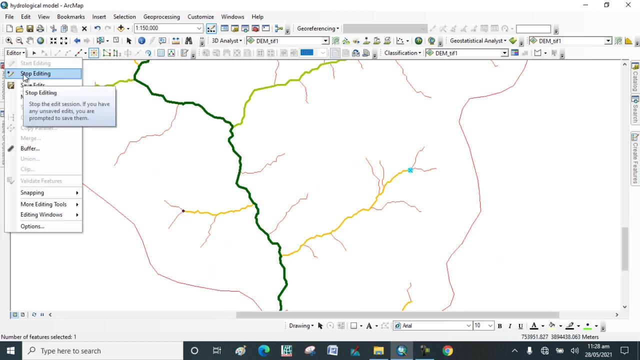 take some point from multi point at the edge of this first order and the second order. so come here and also take point from it, also from there, and also from there and here take some point at. so these are enough. its last point now save, edit and stop the editing. 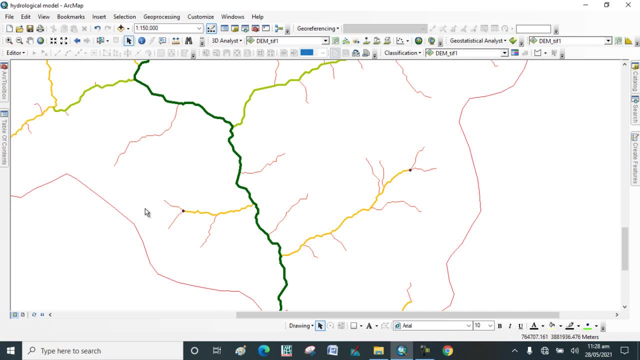 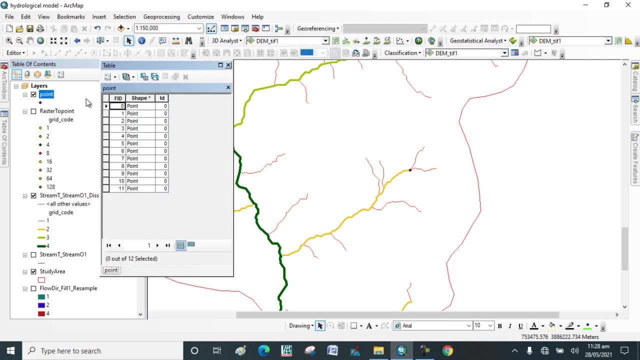 now save, edit and stop the editing. now save, edit and stop the editing. now go to table of the point and give. now go to table of the point and give. now go to table of the point and give the ID number. start editing again to the ID number. start editing again to. 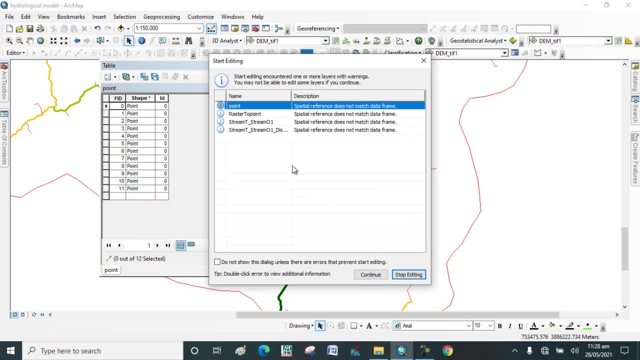 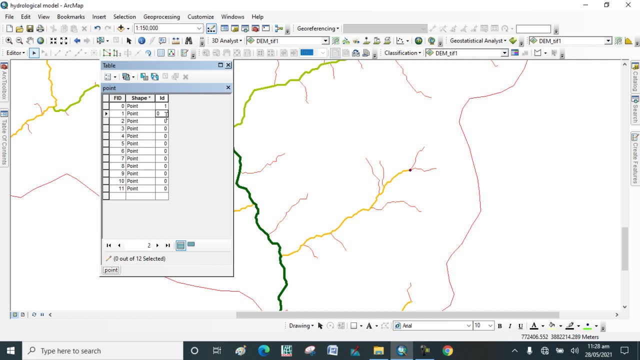 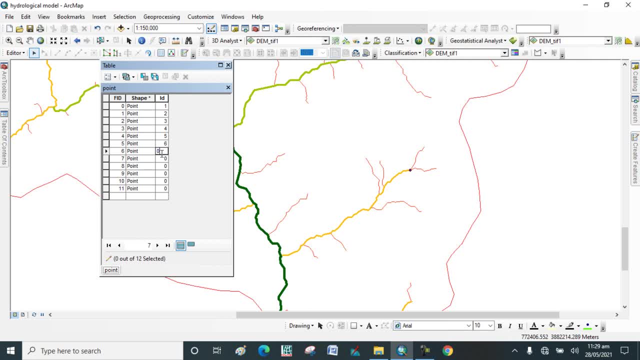 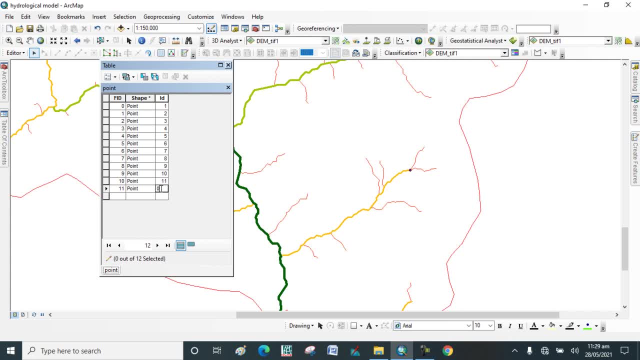 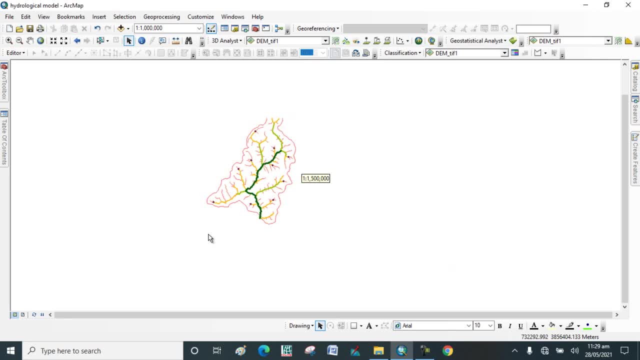 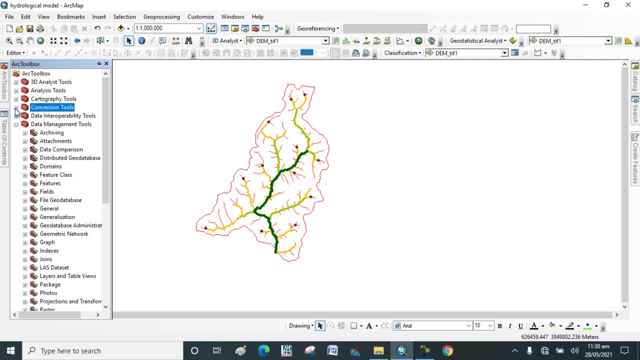 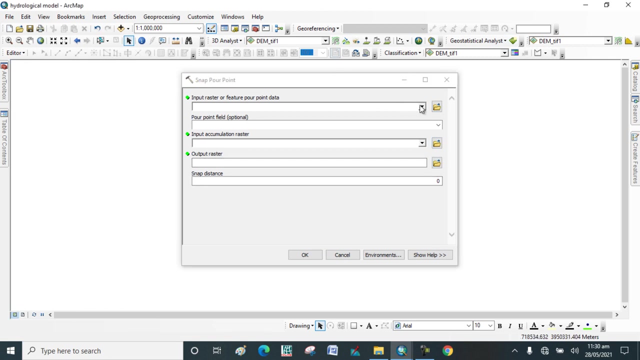 point. okay, continue here, just add number point. okay, continue here, just add number. special analysis tool and go to hydrology tool. hydrology tool: click on snap power point. now we are going toward the hydrological model, so snap power point, click on it and here add the input point, which is known as point or power point. power point field is id and here 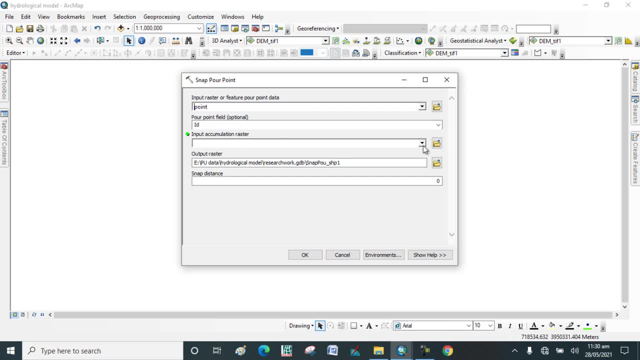 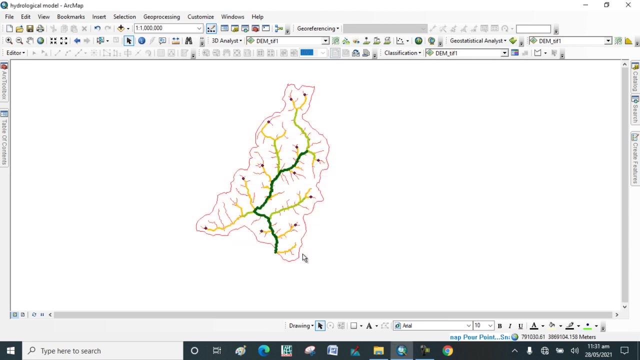 you can add the flow accumulation input, flow accumulation map. this is flow accumulation here. you can then have to snap power point yes and click on ok. now, if you see that we pick the point after that, we will convert it, this point, to the snap power point. if I zoom that here, it will draw the square.